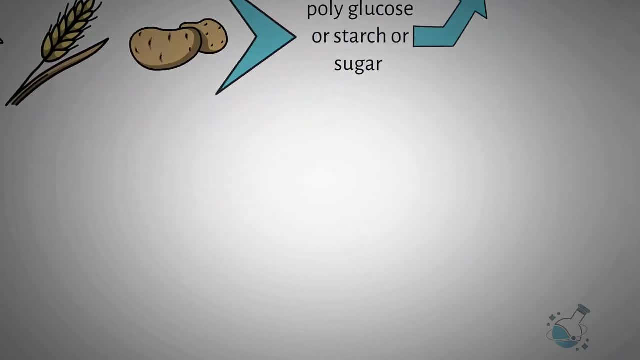 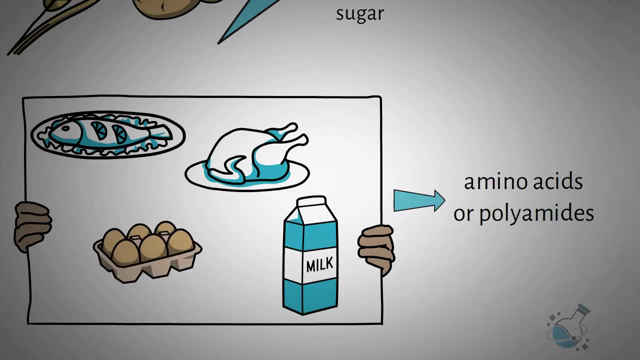 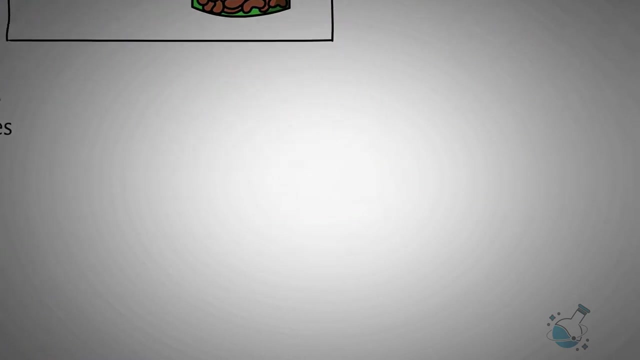 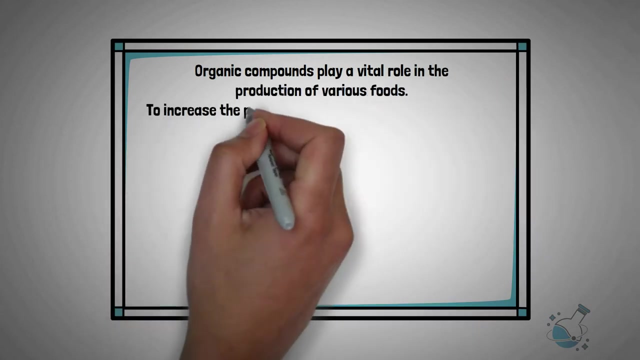 These carbohydrates produce energy inside us The body. Fish, meat, egg, milk, pulse, etc. are good sources of protein, which is formed of amino acids or polyamides. Oils, fats, ghee or butter are in our everyday diet chart. They contain ester lipid. Organic compounds play a vital role in the production of various foods. To increase the production of the crops, we use chemicals like herbicides, insecticides, pesticides, etc. which are mainly organic compounds. 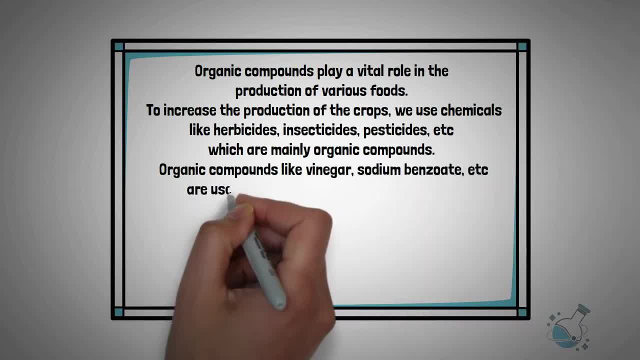 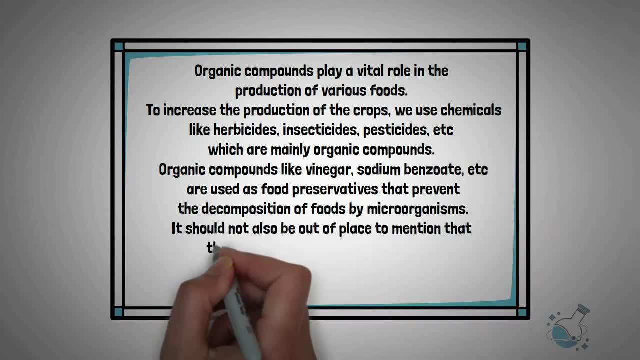 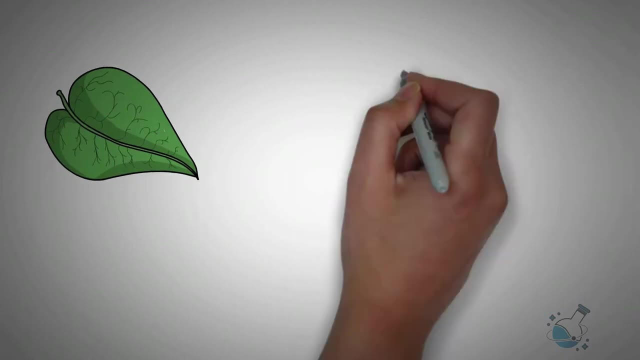 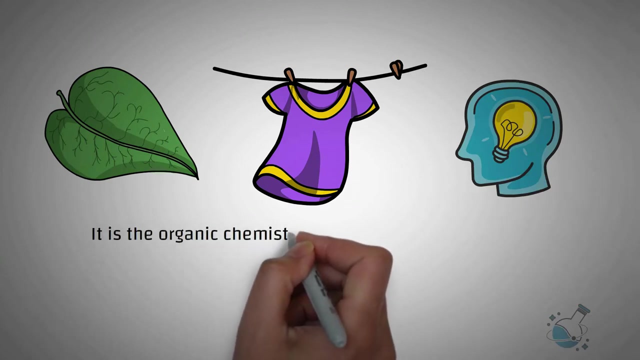 Organic compounds like vinegar, Sodium benzoate, etc. are used as food preservatives that prevent the decomposition of foods by microorganisms. It should not also be out of place to mention that the food colors or sweetening agents are mostly organic compounds. Again, we use coal, natural gas, wood, etc. for cooking food. From wearing large green leaves earned from forest trees to wearing all the modern clothes with a lot of versatile designs, human civilization has become smart enough And it is the organic chemistry which is what we need. 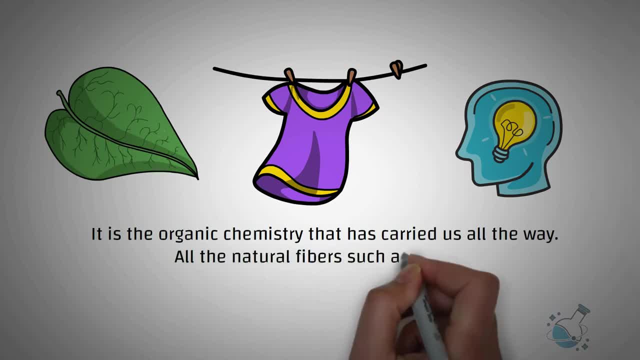 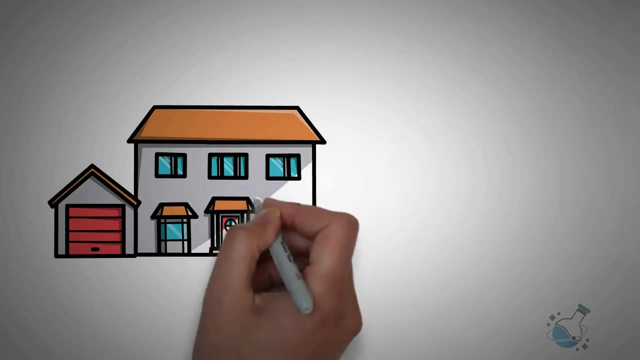 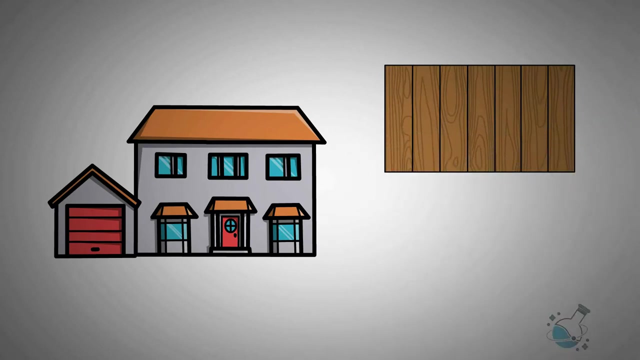 That has carried us all the way. All the natural fibers such as cotton, silk, wool, etc. are nothing but cellulosic materials. Also, synthetic fibers like polyester, nylon, etc. are organic compound polymers. Almost all the materials we use for building a house are organic compounds. Woods we use for making different furniture are compost of cellulose, which is a polymer of glucose. Plastics, paints, varnishes, bamboos, curtains, which modern houses are in fact made of, are organic compounds. 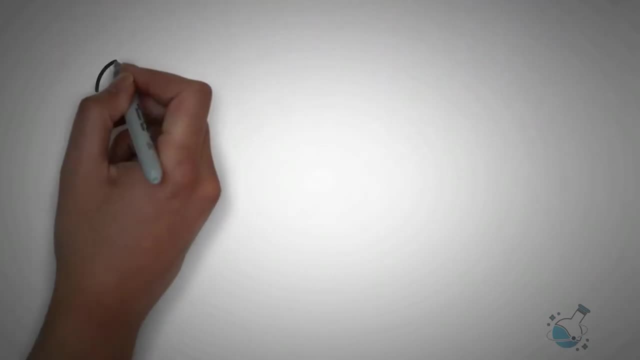 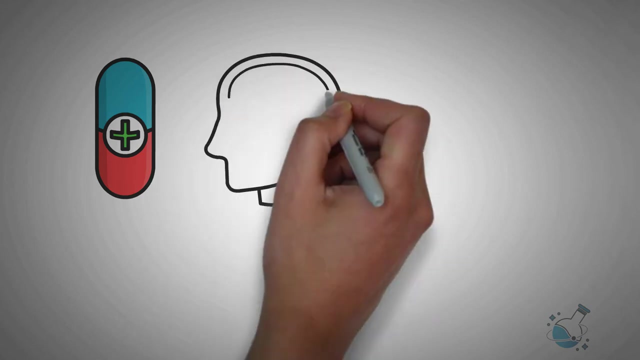 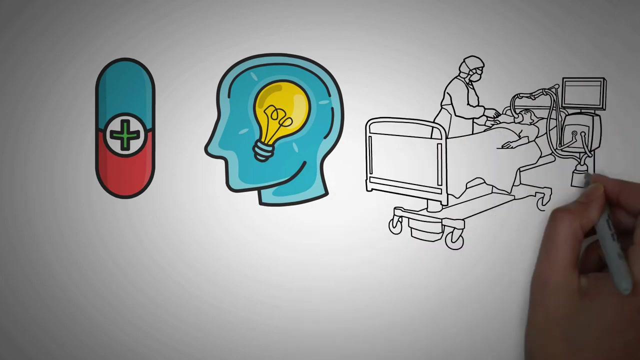 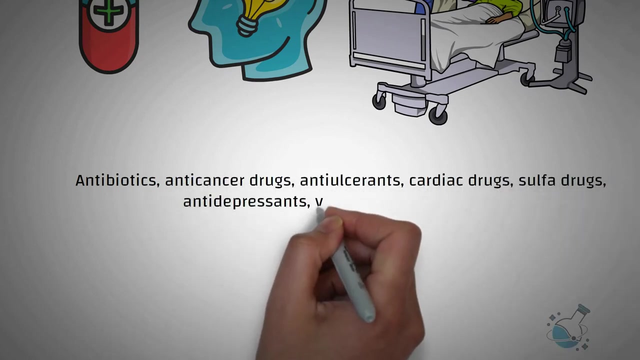 What we cannot complete without are the contributions of organic compounds. We dare not count how many life-saving drugs and medicines have been gifted to human civilization by organic chemistry. Thanks to revolutionary drug discoveries, diseases that once seemed impossible to be prevented or cured can now be faced off quite easily. Antibiotics, anti-cancer drugs, anti-ulcerants, cardiac drugs, sulfa drugs, antidepressants, vitamins, hormones—all are organic molecules.